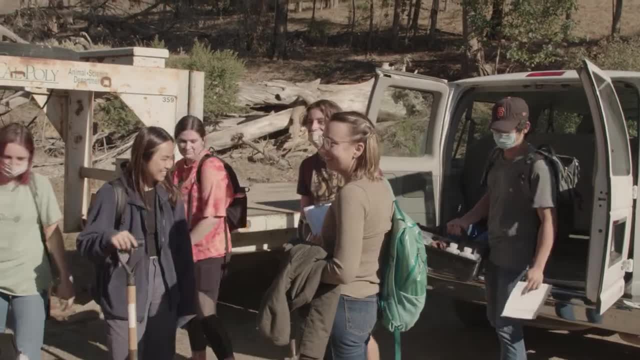 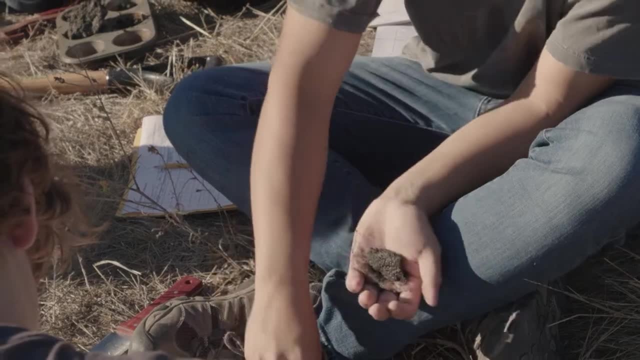 to work outside all the time, right, And so in my classes we literally go out to the field outside every single week and we're out in the field literally getting their hands dirty, learning all these different techniques for recording field observations. 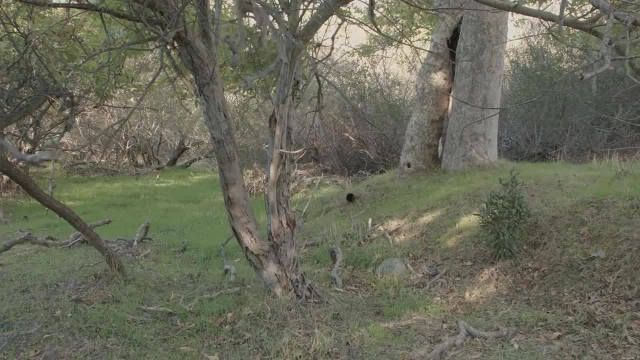 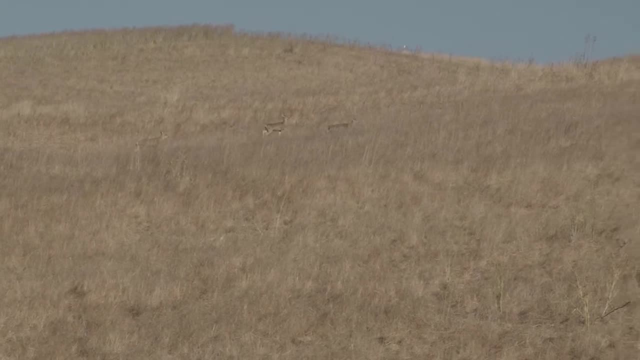 And not just looking at what's in the soil pit, but looking at the entire landscape, looking at geology, the topography, the climate, the vegetation, how it all interweaves together. And that's really what I'm trying to teach my students is how to observe the landscape. 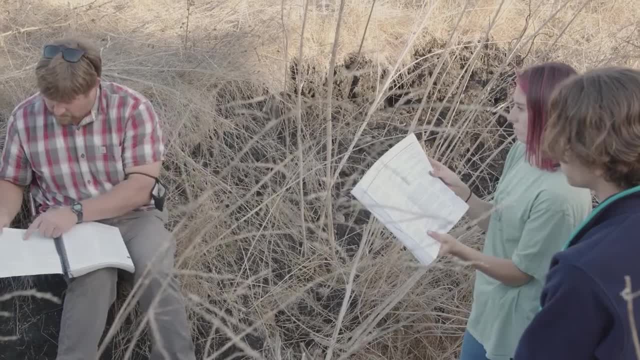 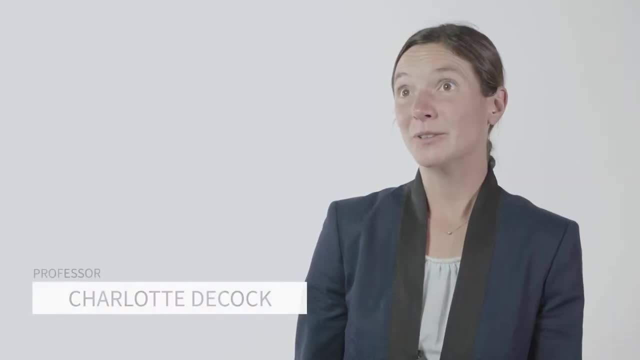 holistically. you know not just what's in the soil- I teach a soils class- but really how all the different parts of the ecosystem interact and interface through the soil resource. The Environmental Earth and Soil Science program at Cal Poly is one of the few programs in 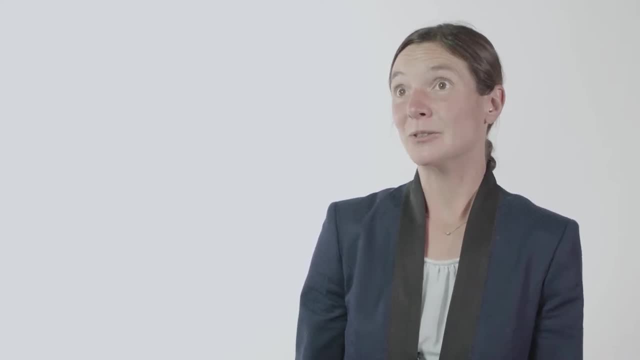 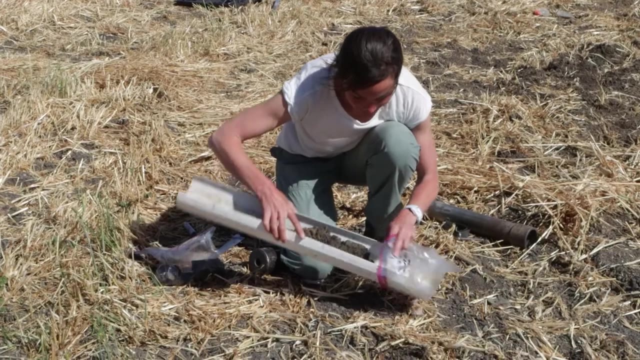 the nation, and not only is it one of the few, it's also got a really good ranking. And so when students come through our program, they are familiarized with all these different instruments, and not only with the instruments but also with all the steps required and sample. 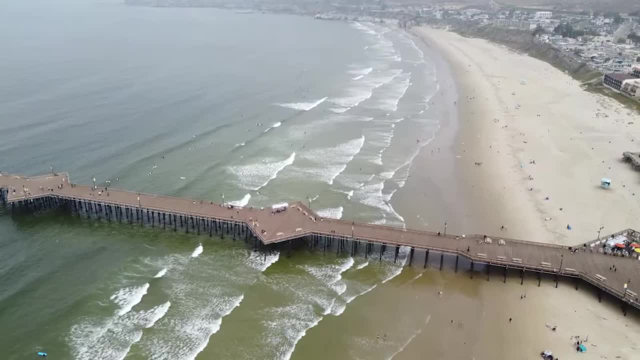 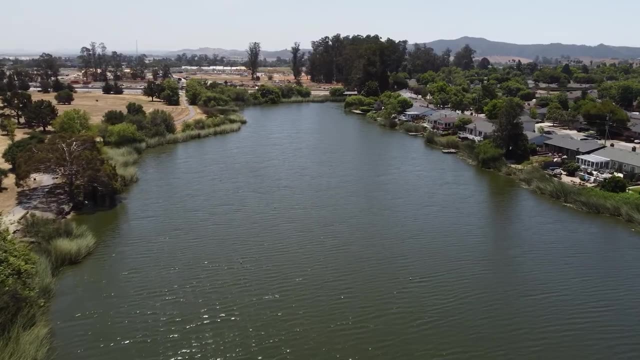 preparation to be able to use that instrument. From my perspective, one of our largest assets is just where we're located. We're located on the beautiful Central Coast, where we have this wide, wide range of different natural ecosystems and resources that are important to protect, but that are also really 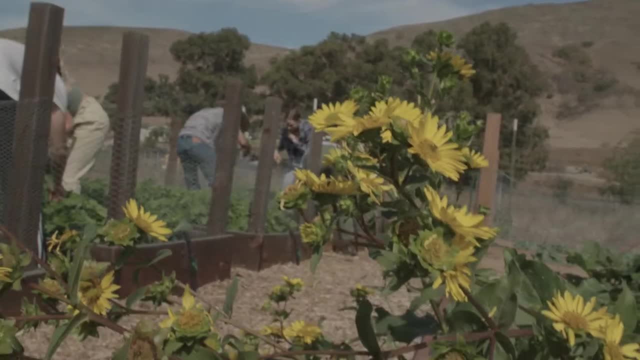 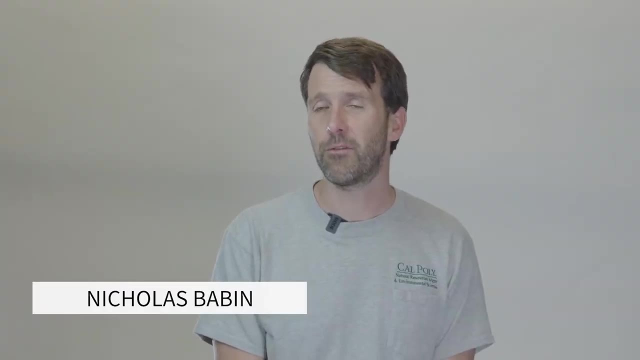 well situated to be learning laboratories for our students. If I were going back to school right now and thinking about a major with a big return on investment, think about forestry and fire sciences And becoming a fire scientist And becoming a professional forester. 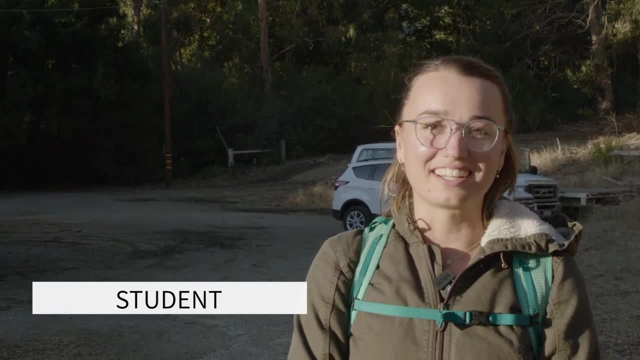 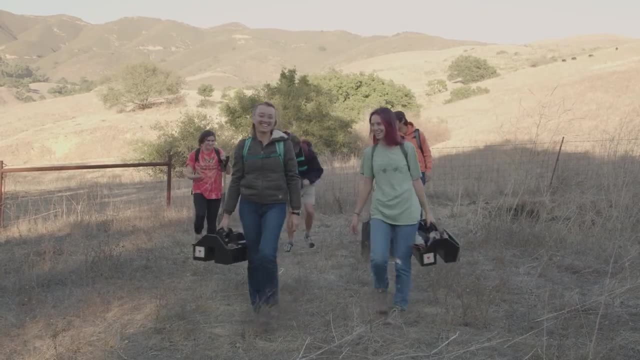 My favorite experience so far has actually been this class. It's been a game changer for how I see the world and how I understand the natural landscape around me. My background is in biology and I don't know that much about the soils, which are a key. 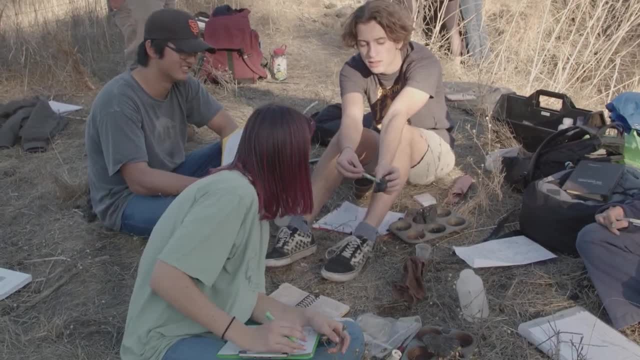 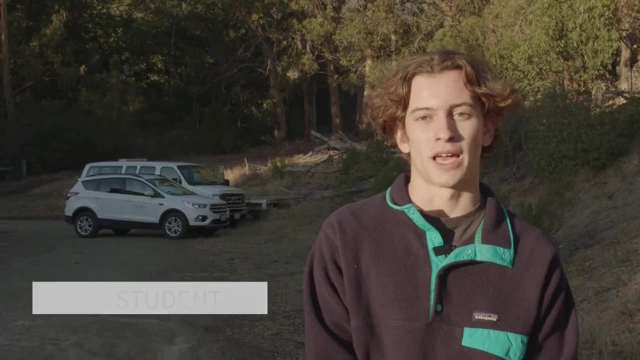 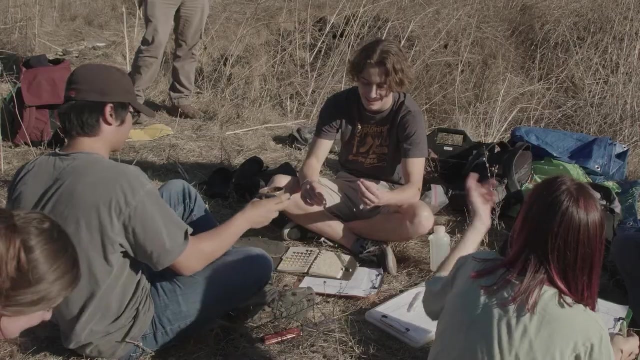 part of every ecosystem, And beginning to understand these soil processes has totally changed my understanding of the natural world. Every week, three to four times a week, I get to go outside And actually get hands-on activities in small groups, like a six-person lab with one professor.